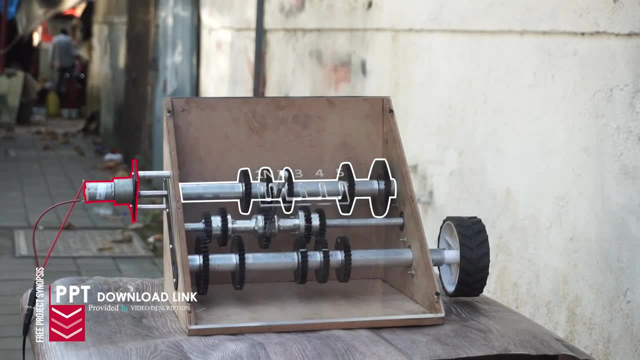 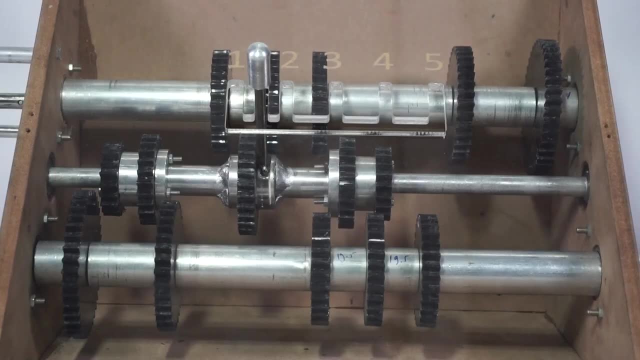 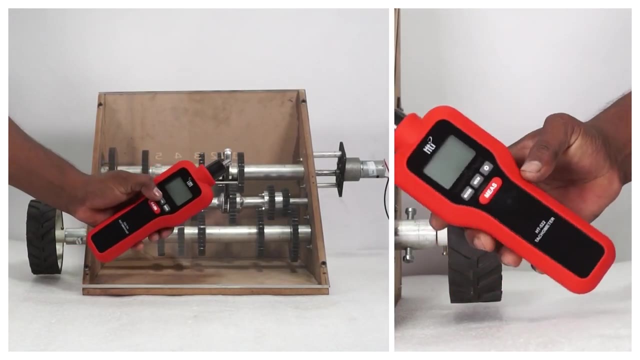 It has a DC motor which is connected to the topmost shaft. This DC motor is used to act as the acceleration of the vehicle or the engine RPM. So now let's change the gears. So now let's switch to the first gear. We will now be using a tachometer to note the changes in wheel RPM, the output RPM of the wheel, each time we change the gear. 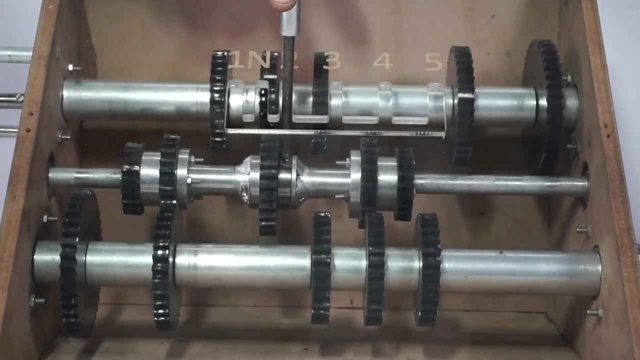 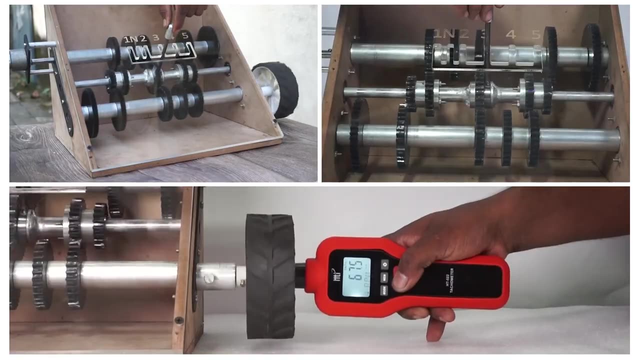 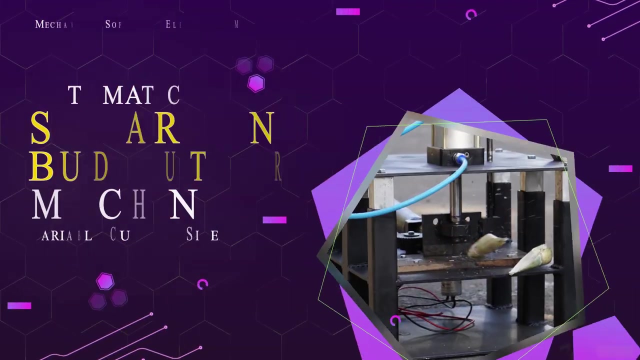 Let's switch to the second gear. You can see the changes in the RPM of the wheel in the tachometer. We now switch to the third gear, Switching to fifth gear. This is how the system works. Automatic Sugarcane Bud Cutter Machine. 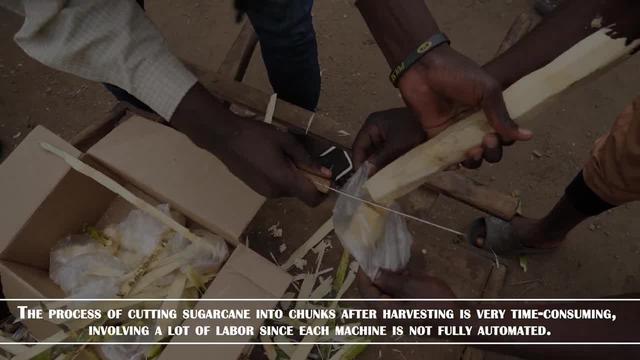 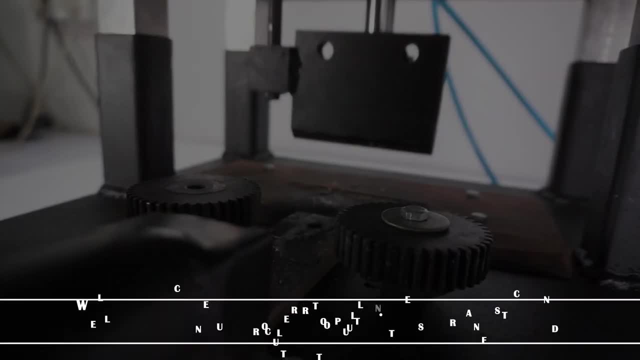 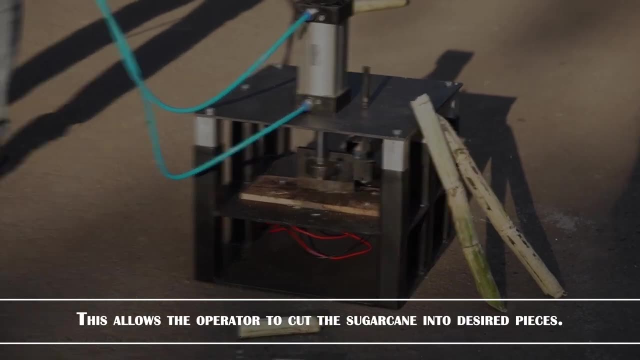 The process of cutting sugarcane into chunks after harvesting is very time consuming, involving a lot of labour, since each machine is not fully automated. Well, this machine uses rollers to pull in the sugarcane stick and a cutter to cut it. This allows the operator to cut the sugarcane into desired pieces. 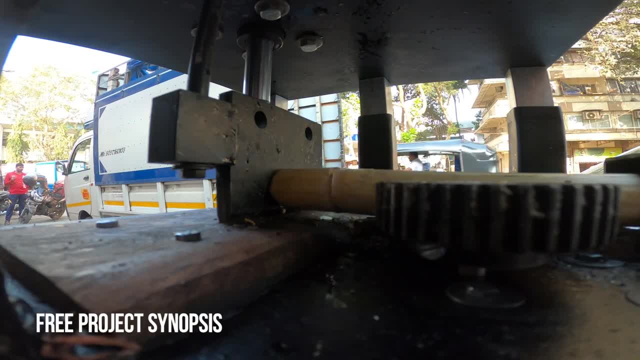 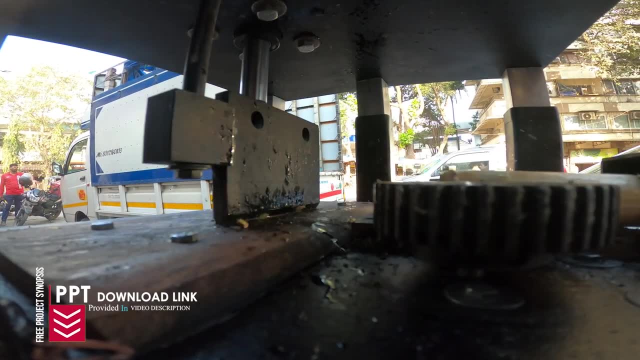 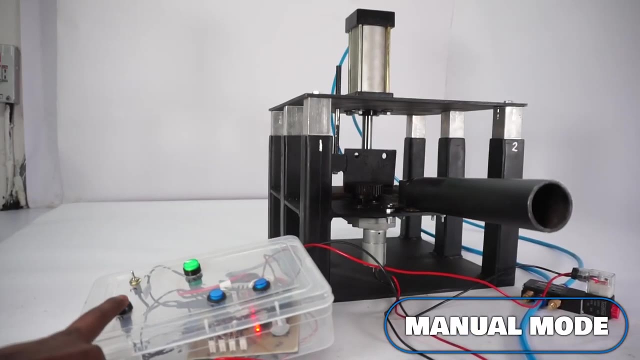 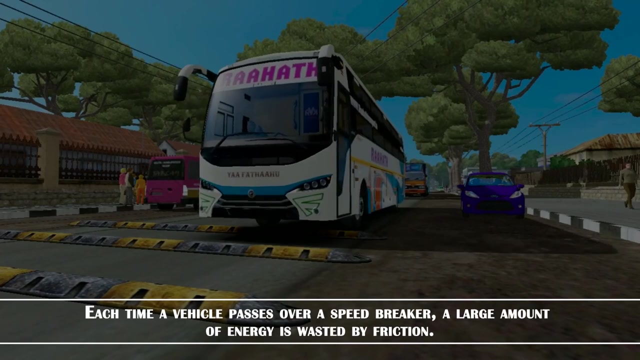 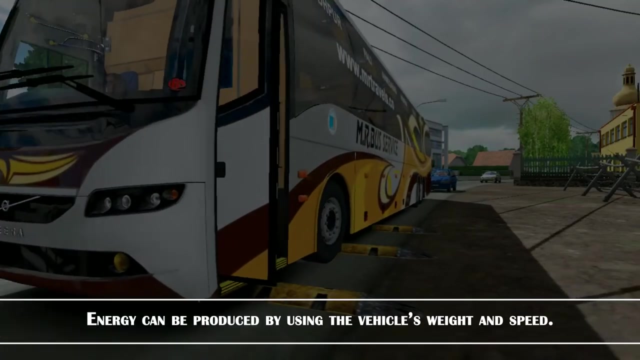 Power generation using speed breakers. Each time a vehicle passes over a speed breaker, a large amount of energy is wasted by friction. Energy can be produced by using the vehicle's weight and speed, So here we propose a smart speed breaker that generates power. 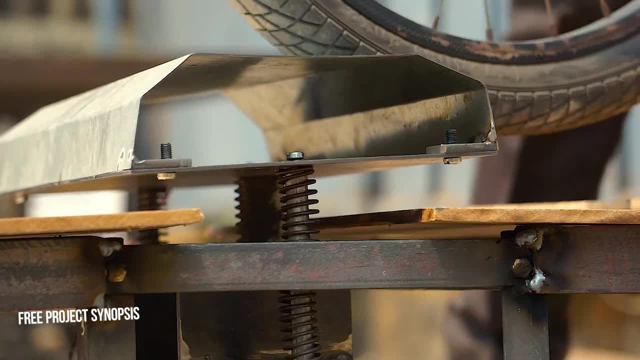 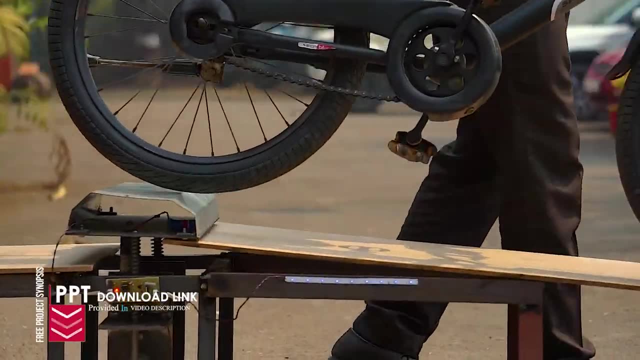 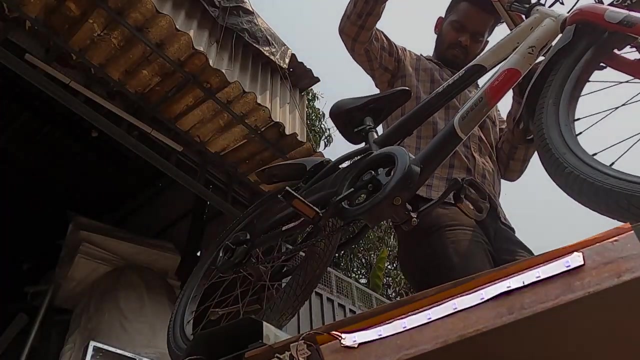 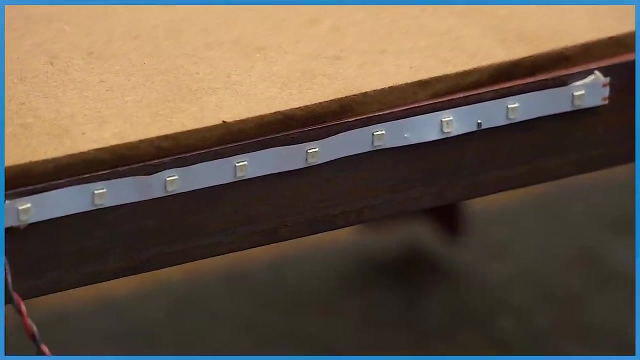 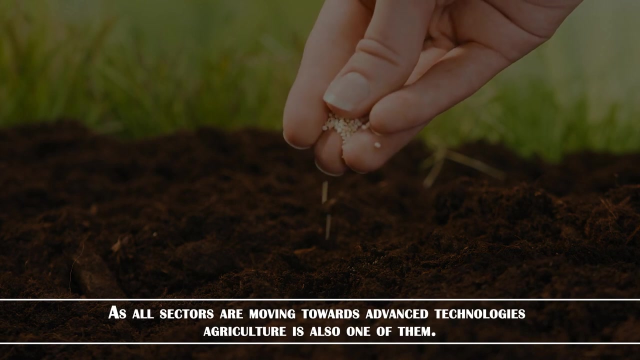 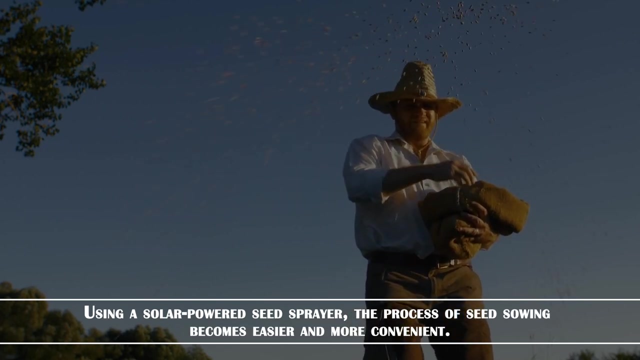 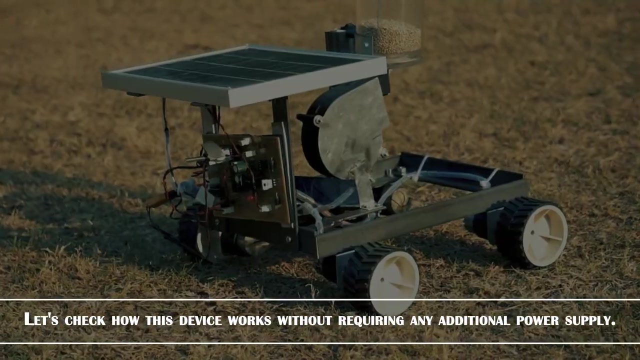 Elevator, L programming machine, Sample Machine, Transformer. sectors are moving towards advanced technologies. agriculture is also one of them. Using a solar powered seed sprayer, the process of seed sowing becomes easier and more convenient. Let's check how this device works without requiring any additional power supply. 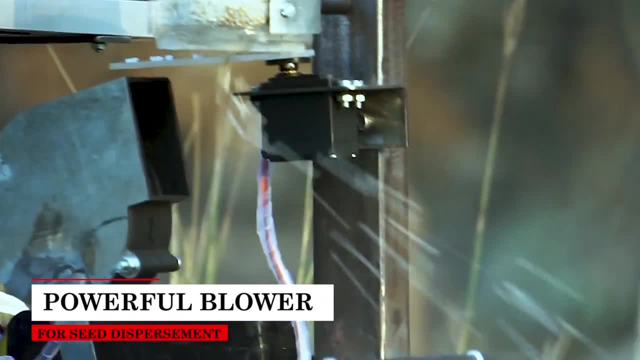 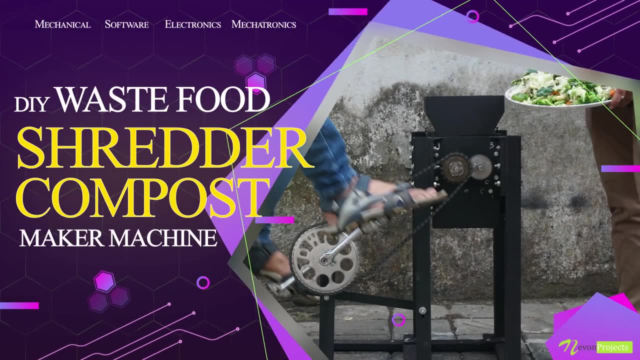 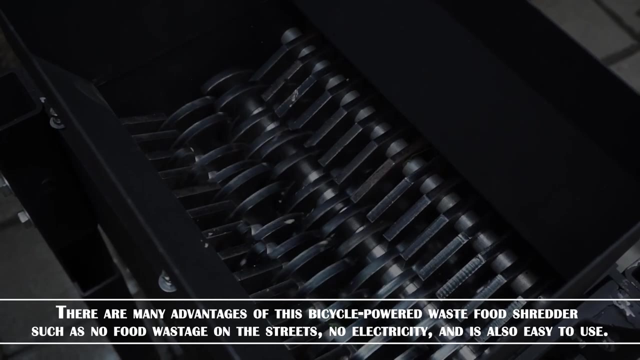 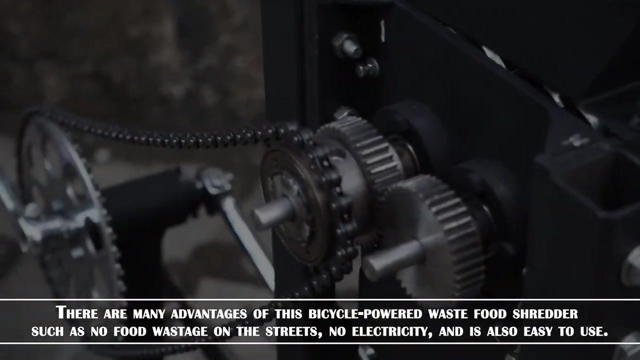 DIY Waste Food Shedder- Compost Maker Machine. Shedding of waste food speeds up the decomposition process. There are many advantages of this bicycle powered waste food shedder, such as no food wastage on the streets, no electricity, and it is also easy to use. 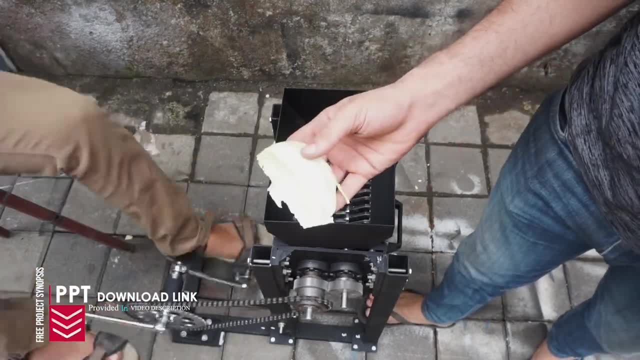 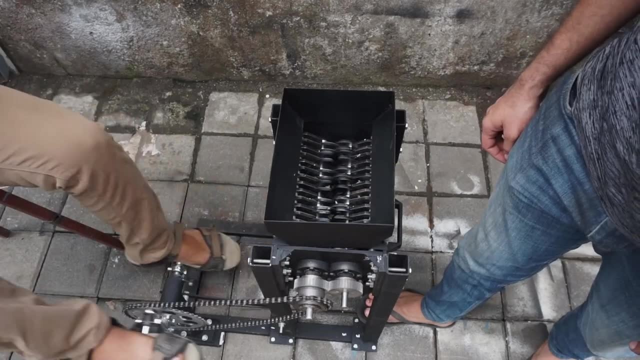 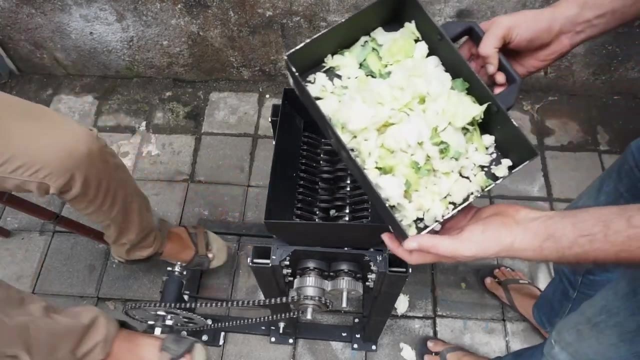 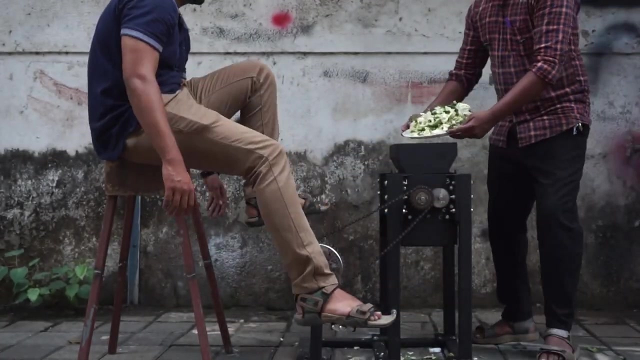 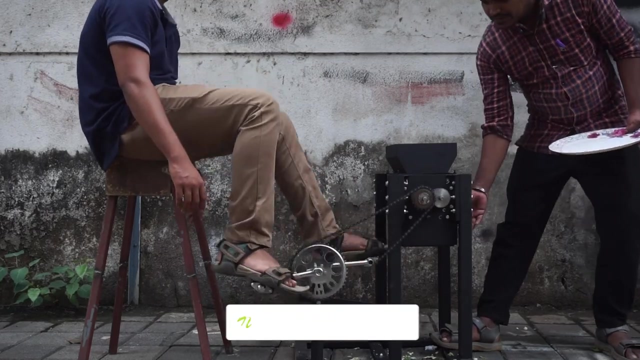 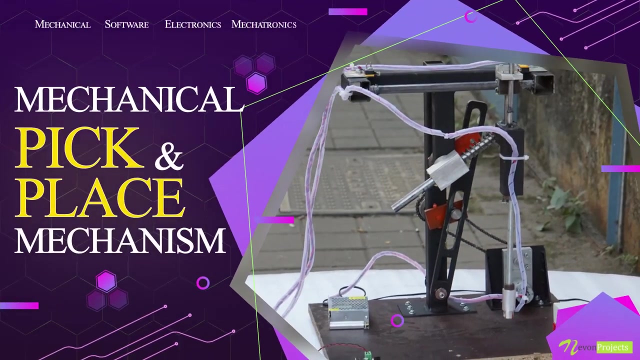 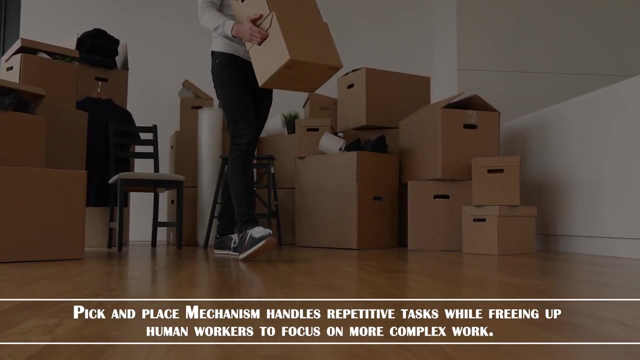 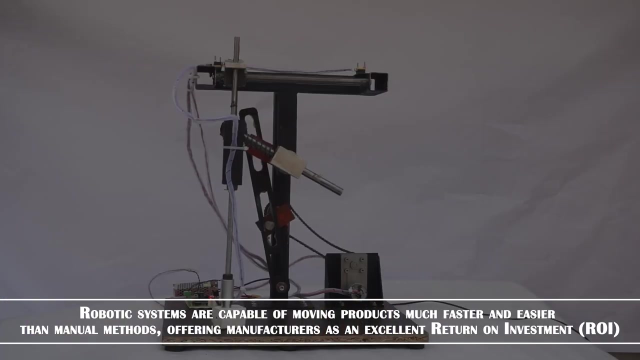 Power supply. Mechanical Pick-and-Place Mechanism. Pick-and-Place Mechanism handles repetitive tasks, while freeing up human workers to focus on more complex work. Robotic systems are capable of moving products much faster and easier than manual methods, offering manufacturers an excellent return on investment. 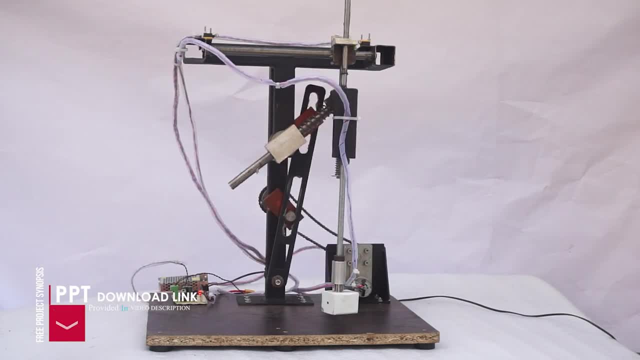 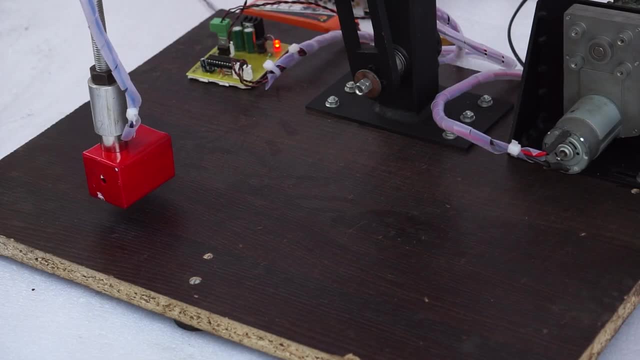 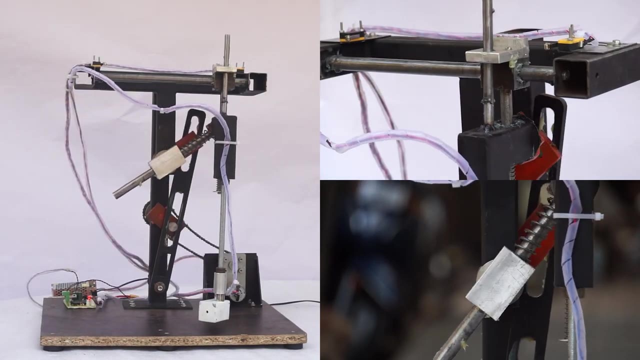 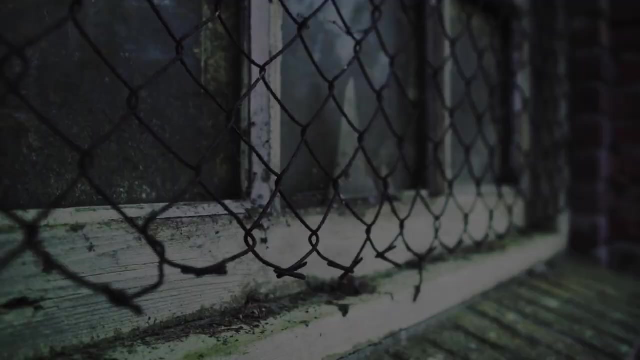 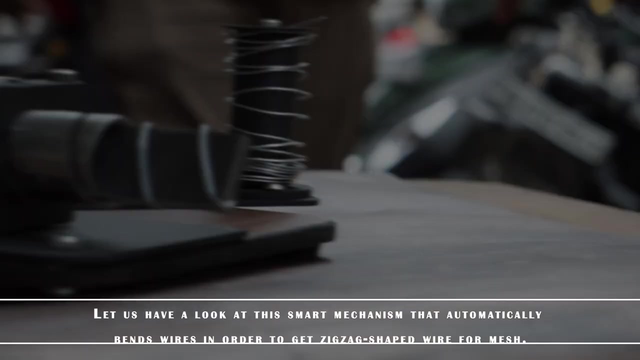 Chain Link via Mesh Making Machine. Preparing zig-zag shaped wire is a quite challenging task and cannot be done using basic mechanics. Let us have a look at this smart mechanism that automatically bends wires in order to get zig-zag shaped wire for mesh. 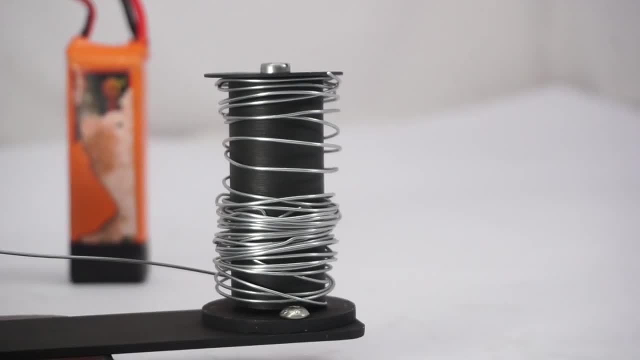 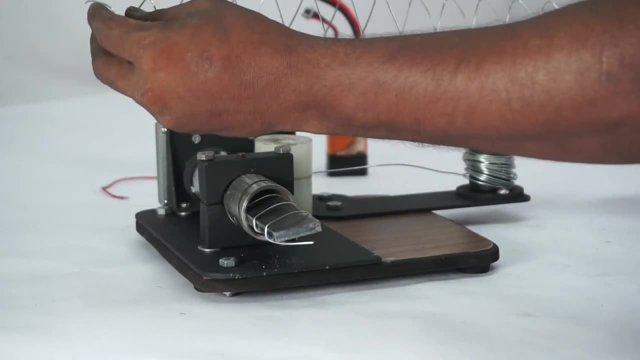 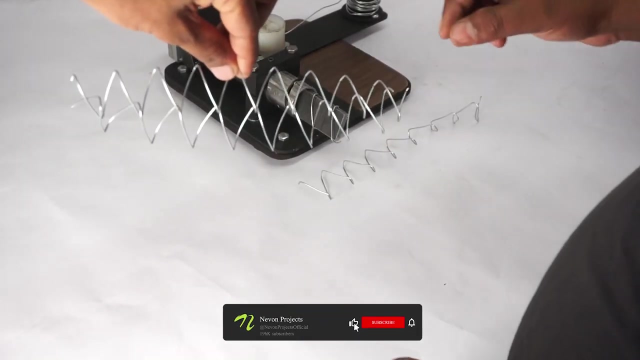 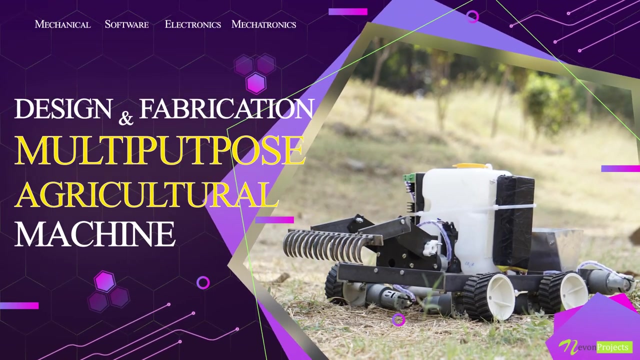 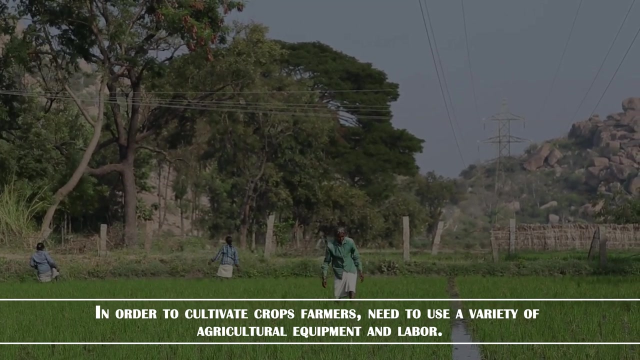 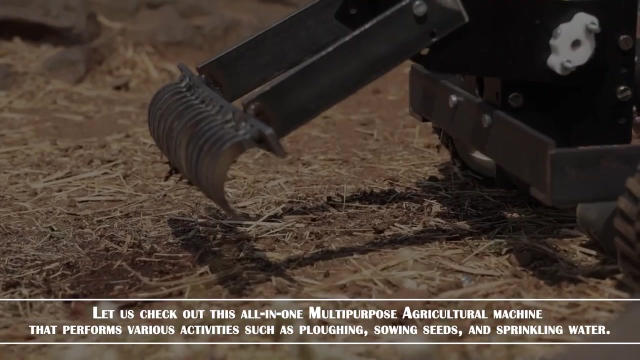 Design and Fabrication of Multi-Purpose Agricultural Machine. In order to cultivate crops, farmers need to use a variety of agricultural machinery. Let us check out this all-in-one multi-purpose agricultural machine that performs various activities such as ploughing, sowing seeds and sprinkling water. 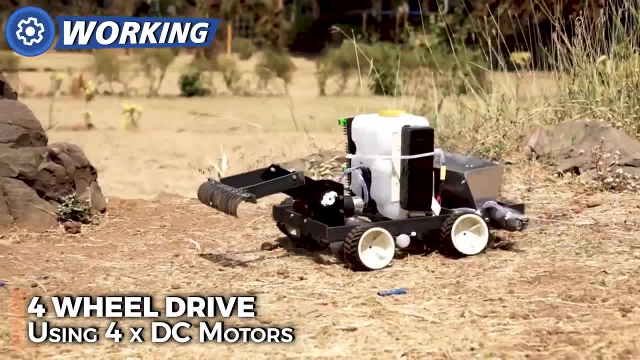 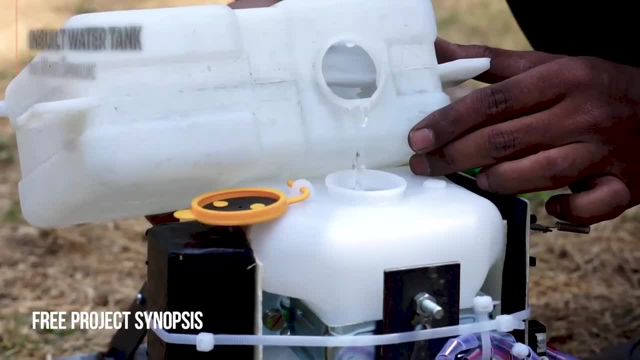 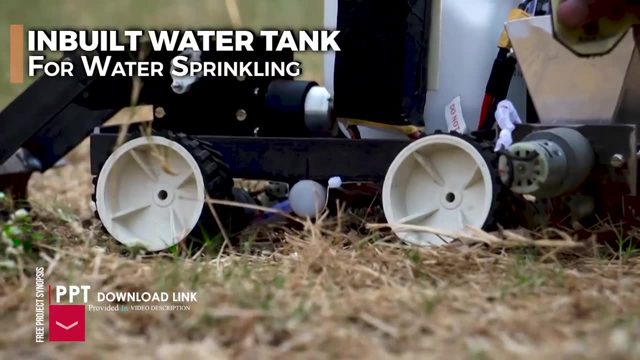 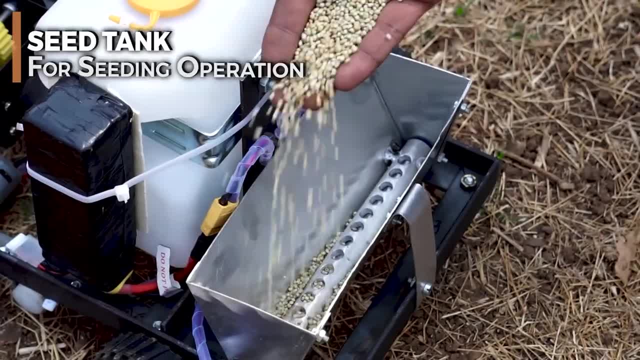 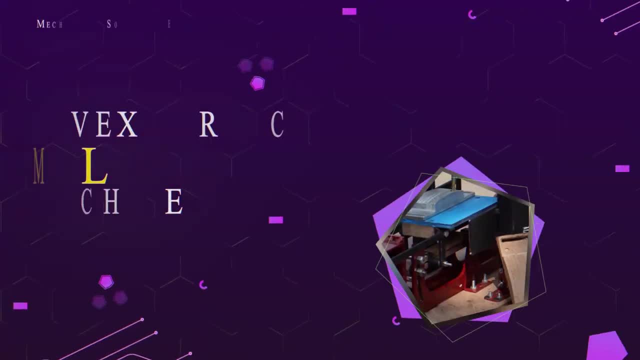 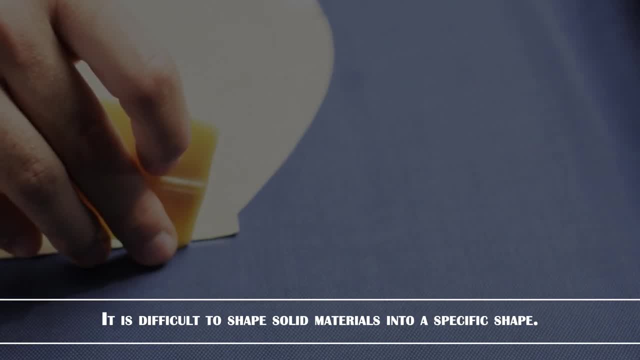 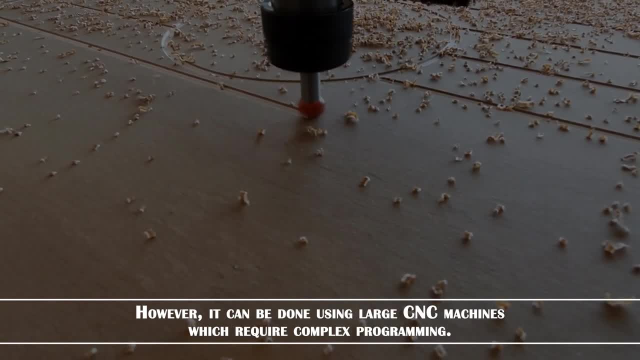 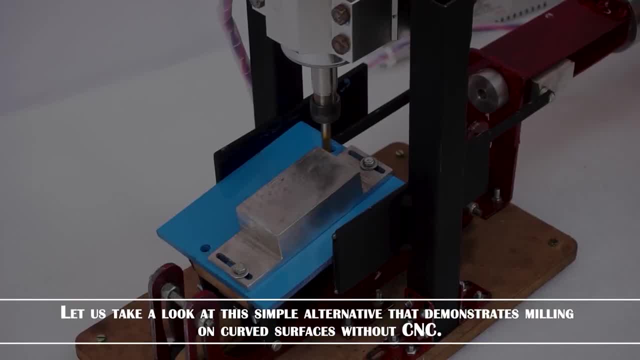 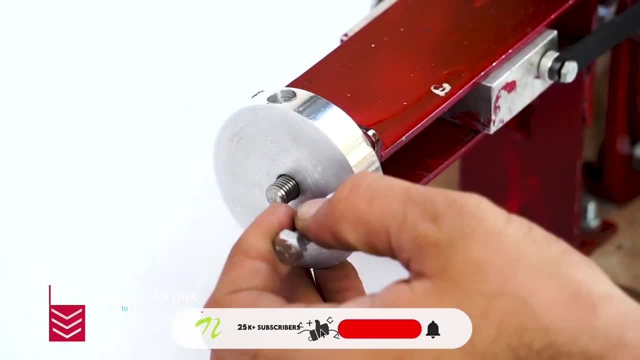 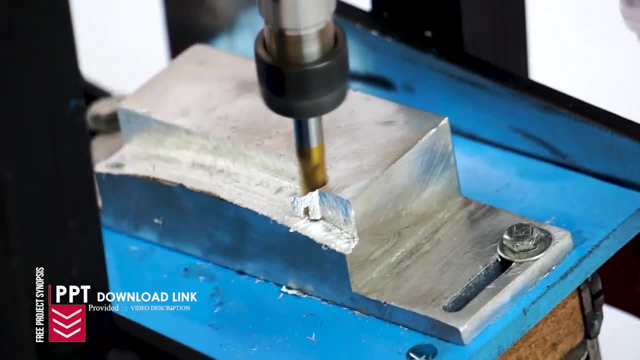 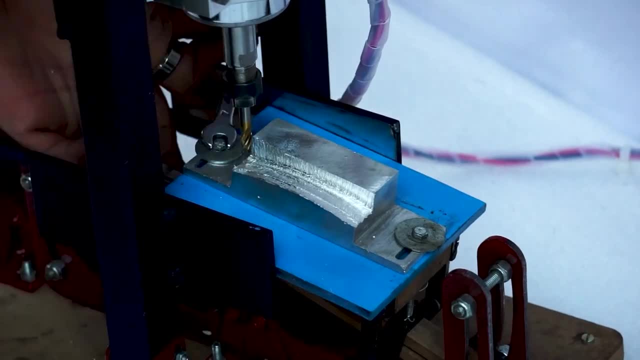 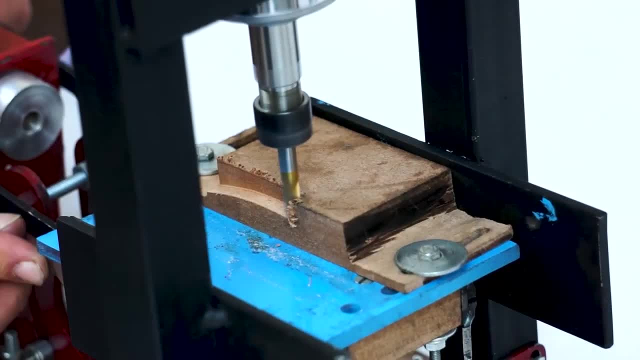 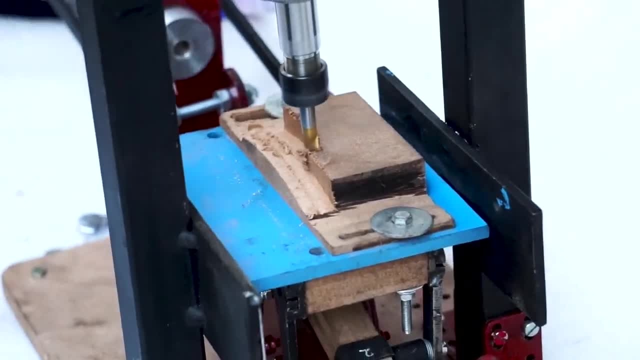 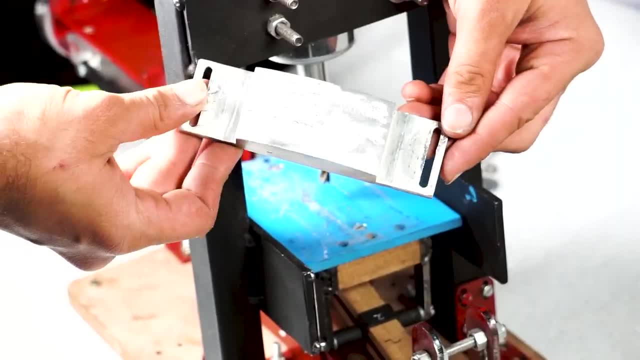 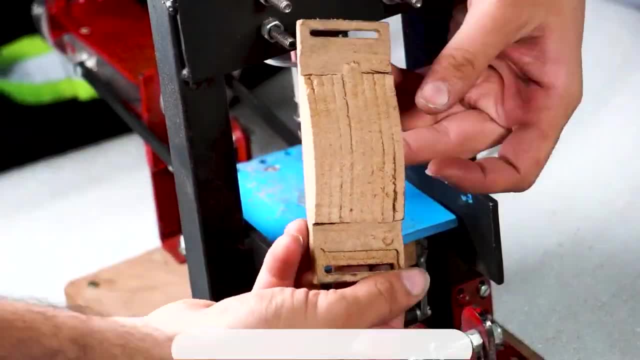 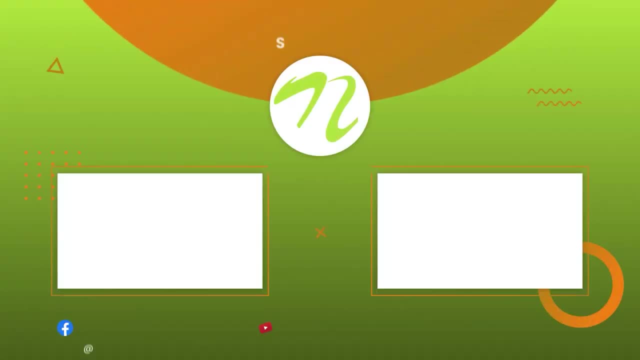